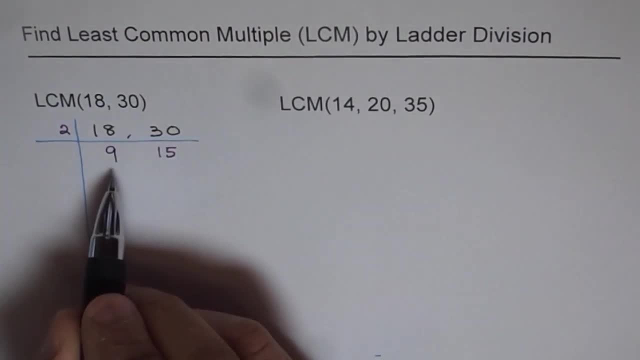 2, you get 15.. Now we see, 3 is a common factor between the 2. So let's divide it by 3.. So we'll go and get the answer down. There we go. so that would be 13.. So if minus a Co souvent s Bq-vo, Frances, eoч, vbIrgLV, sO, J, oEV-lV�ZJs Li. 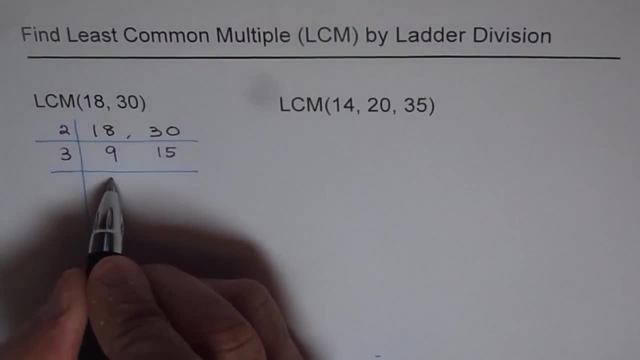 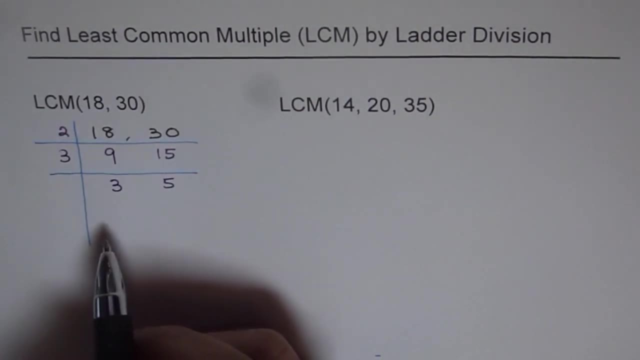 So we get: 3 goes 3 times in 9 and 5 times in 15.. Now we have all the prime factors here: 2, 3, 3 and 5. That gives us the least common multiple between the two given numbers. 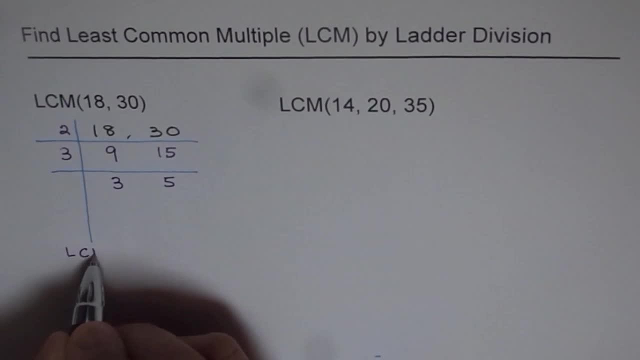 So we can get our answer, as LCM equals 2, product of these prime factors. So they are 2 times 3 times 3 times 5.. And now you can multiply them and get the answer. Multiplication- well, the most convenient is 5 times 2, first right. 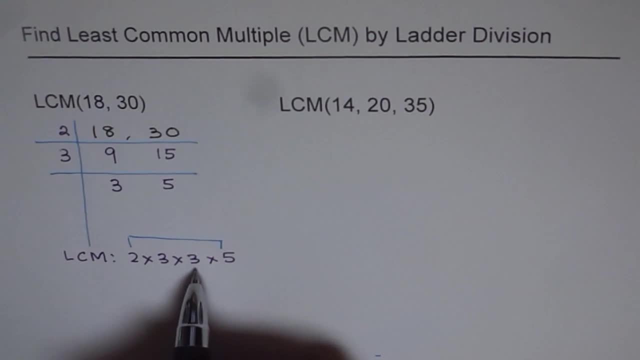 That gives you 10, right. And then 3 times 3 is 9.. So you get 10 times 9 and that is 90. So the LCM for 18 and 30 is 90.. Now think about writing multiplications. 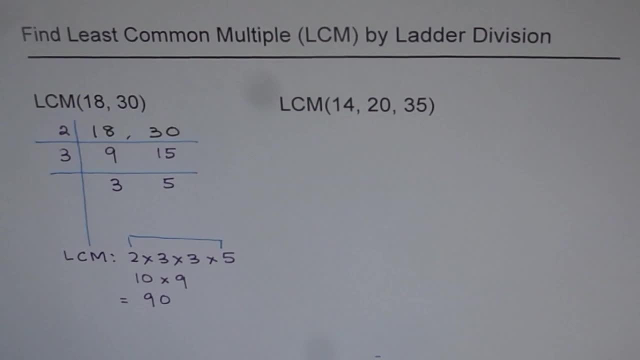 Multiples of 18 and 30 and then getting the answer. That will be very time consuming. So this method of letter division is very efficient And it can be applied to 2 or more numbers. Now let's see how to apply this method with 3 numbers. 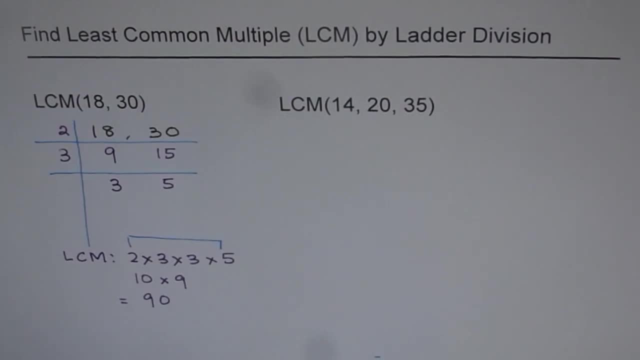 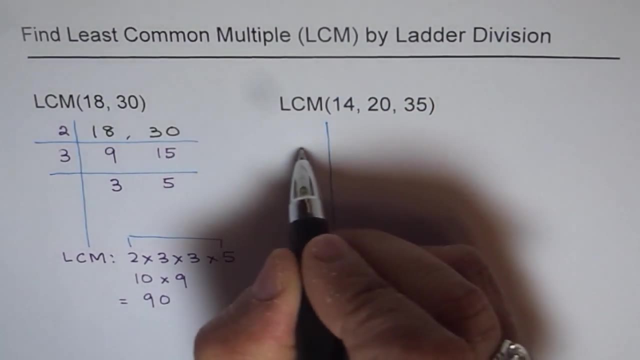 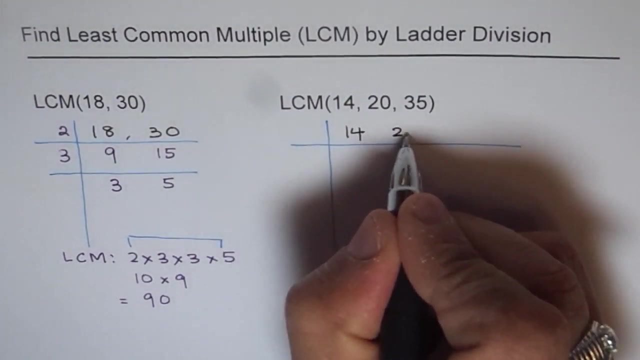 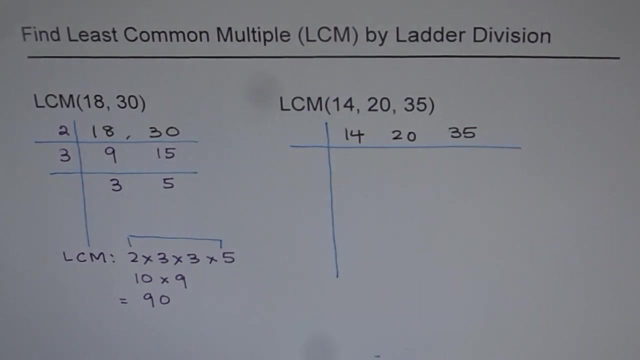 So let's try to figure out what is the LCM of 14,, 20 and 35. So we will again make a division column here and list our numbers. The numbers for us are 14,, 20 and 35. Try to find prime numbers which can divide into at least 2 of them. to start with, 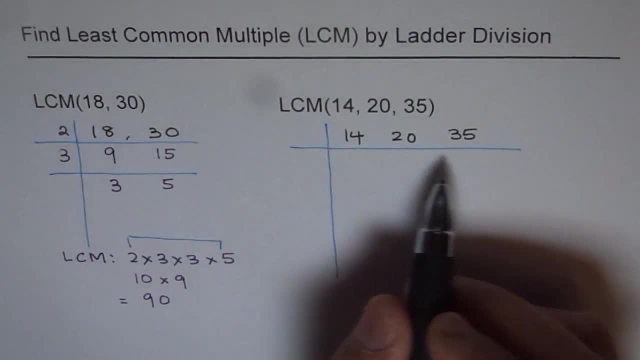 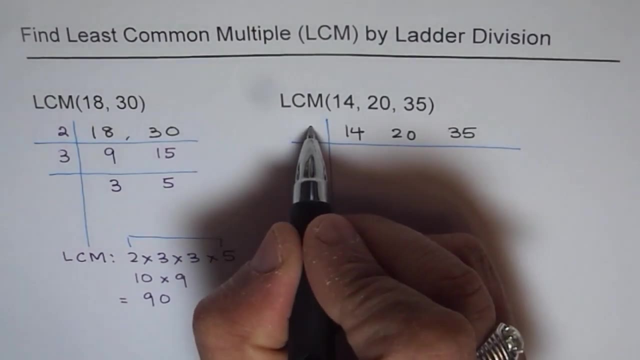 Or all 3 of them, right? Well, we really don't have any number which could divide into all 3 of them, right? So let's start with 2 of them. So the prime number 2 is a good number to start with, always. 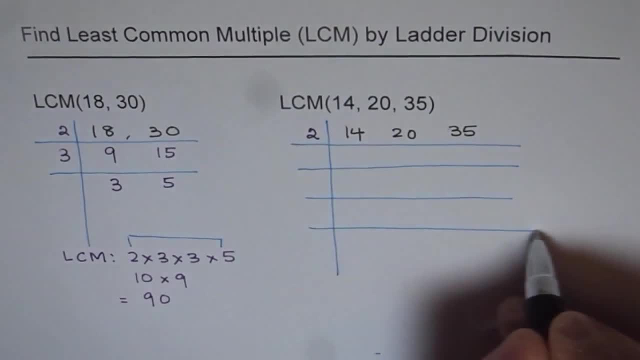 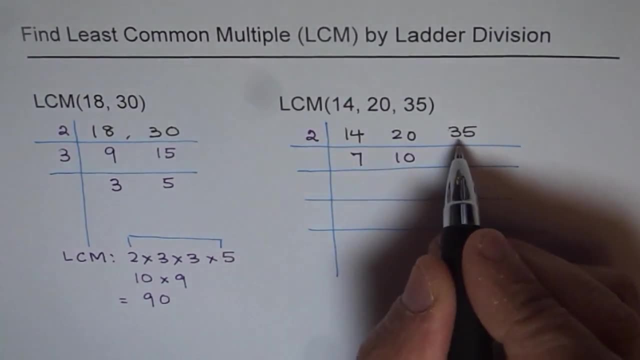 Now, if you divide by 2, what do you get? 2 goes 7 times in 14, 10 times in 20, and 2 is not a factor of 35. So in this case, just copy the number 35 as such. 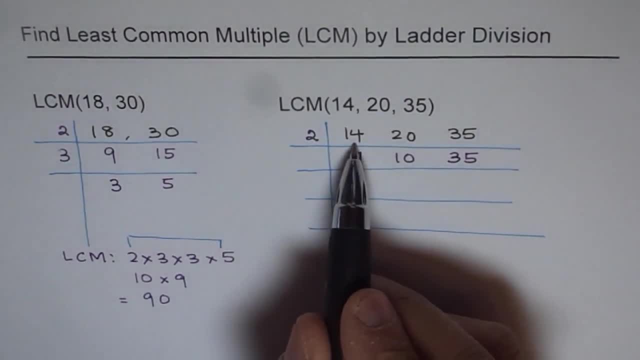 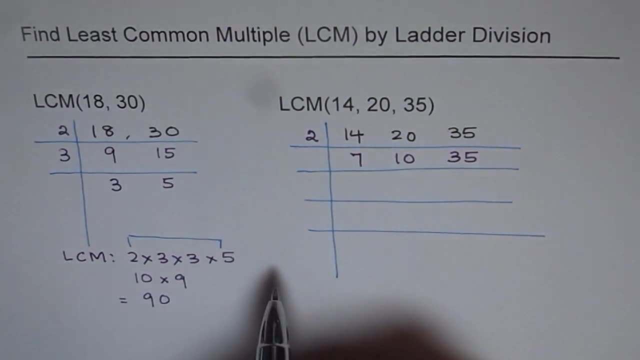 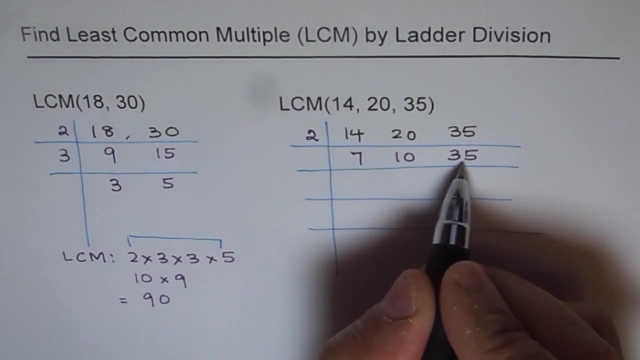 Correct, But at least we factored out 2 from 14 and 20 and we are a step closer to the least common multiple. Do you understand? That is the concept. Now the common factors between these could be 7.. 35 is 7 times 5.. 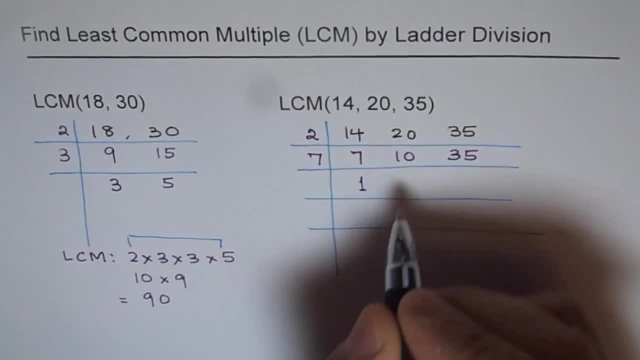 So we can divide it by 7.. 7 goes 1 time. 10 does not have 7 as a factor, So you cannot divide 10 by 7.. So we will copy the composite number 10 as such. 35 goes 5 times. 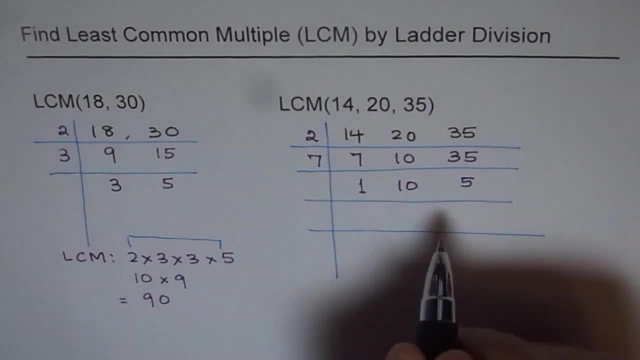 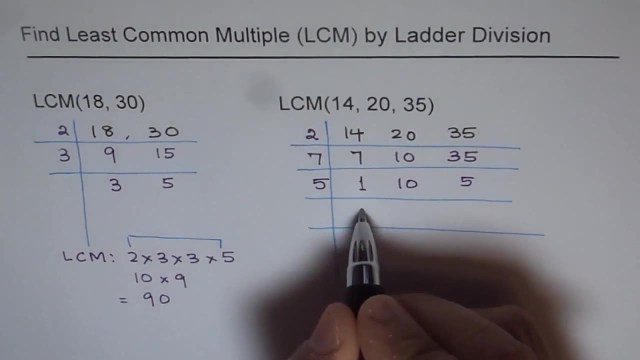 7 times 5 is 35. Now you can see that we have 10 and 5. Which has a common factor of 5.. So let's divide by 5.. Retain 1. here, 10 goes 2 times and 5 1 time. 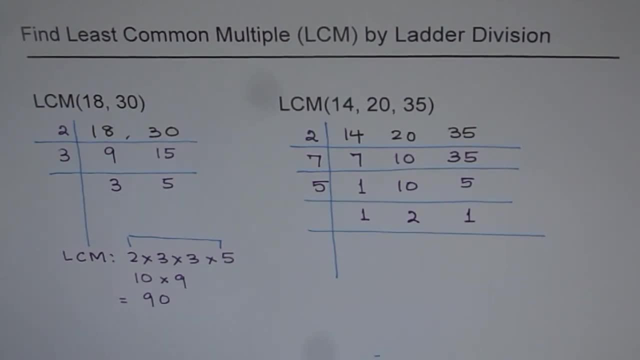 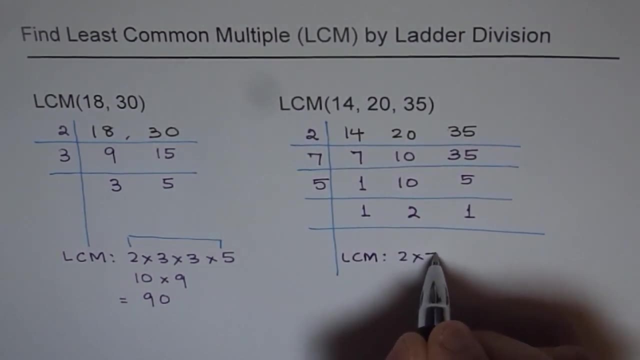 So now again, we have all prime numbers with us. LCM is product of these prime numbers. We can write LCM as 2 times 7 times 5 times 2.. So write down all the prime numbers. 1 you could have written. 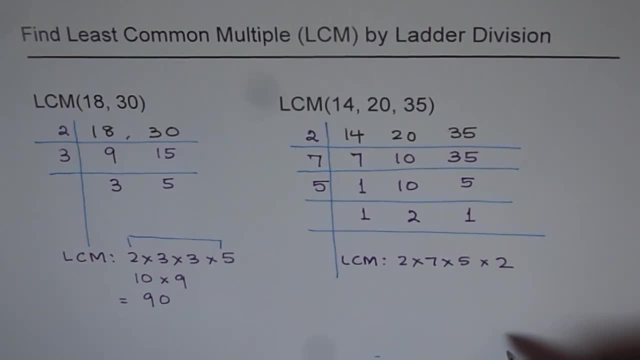 Remember one thing: 1 truly is not a prime number. Prime numbers are numbers which have at least 2 factors. In fact, they have exactly 2 factors 1 and number itself, 1, has only 1 factor: 1 and 1.. 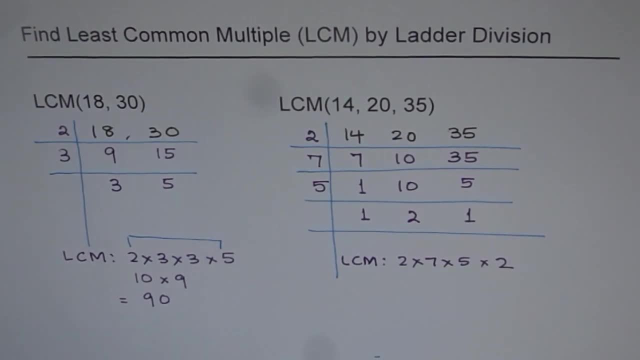 That is just 1 number, And even otherwise, multiplying by 1 gives you the same number. Now let's multiply them. So good order to multiply is: 2 times 7 will be 14. And 5 times 2. 10.